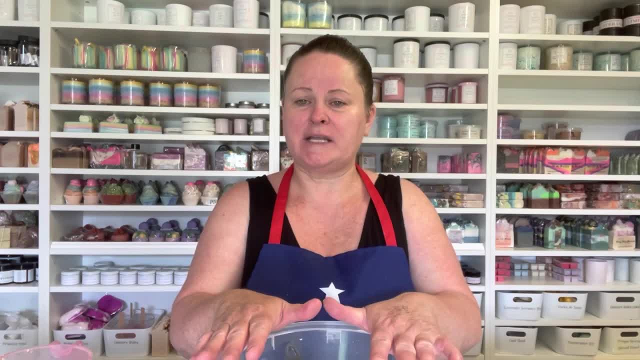 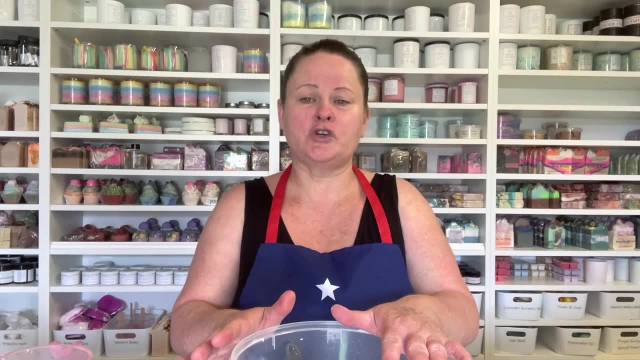 and also the water, because that is our water content that we're using for the baby one. Of course it's for a baby, so we are not going to be adding in any soap. So we're going to be adding in, and we are also not going to be adding in any colors. We're going to leave it totally natural. 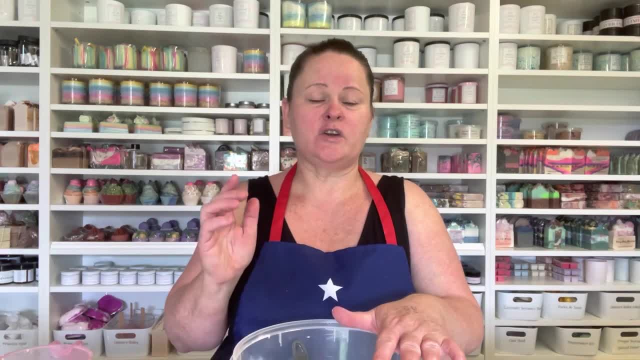 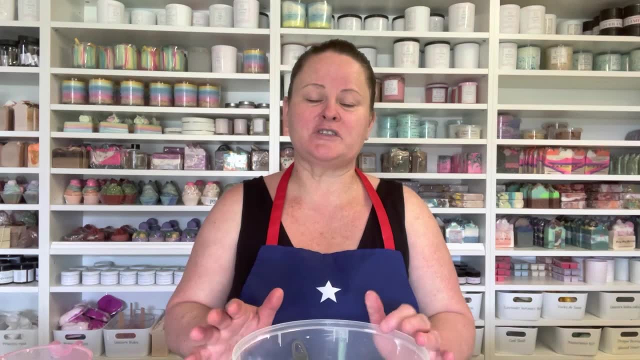 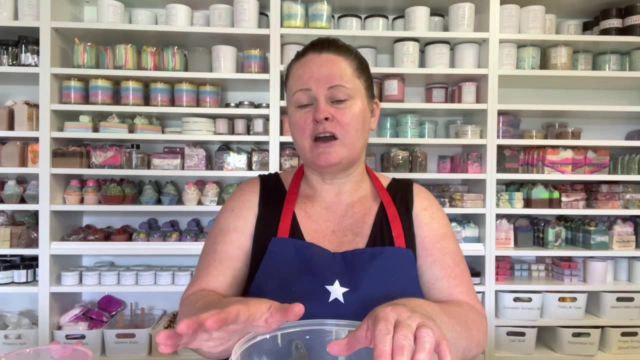 and these are the only products that are going to be in it. So it'll be lye, shea butter and olive oil, and that is absolutely it, And it will be really gorgeous. but do remember, because it is a much softer recipe, this one does need to sit there and rest for a couple months at least. I leave mine. for about 10 months, but usually within five or six months you will be able to use it, But I just give it a little bit more cure time. So if you're going to be using it for a baby, you're going to need to make sure you're always on the go and that you're always looking at your inventory. At the moment, I'm 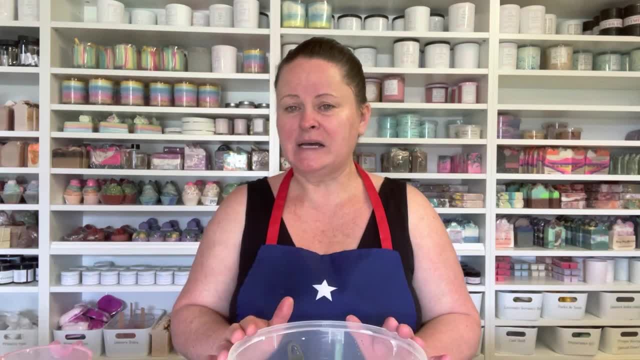 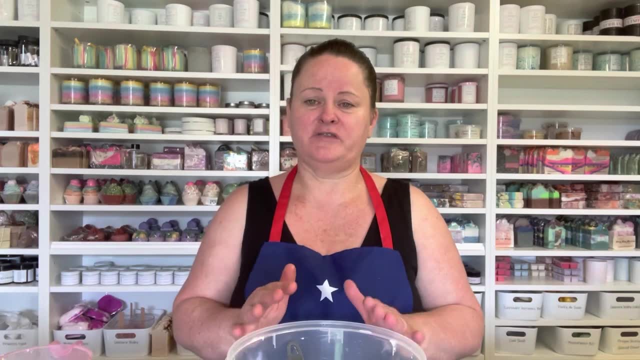 running really low. I do have some that will be ready in December, but you know, generally you need to just keep going with this. So I'm rolling it around. So obviously, if you get down to a few hundred bars, you'll need to make more, because you need to give that sort of four to six month. 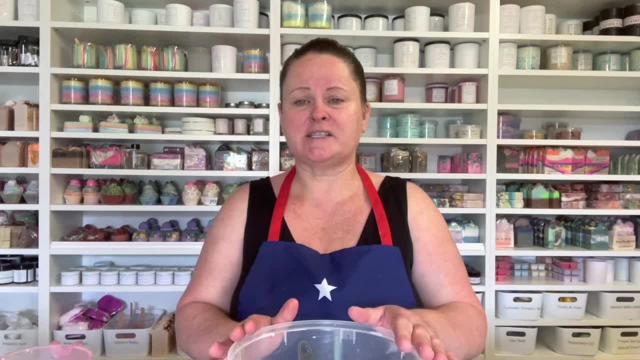 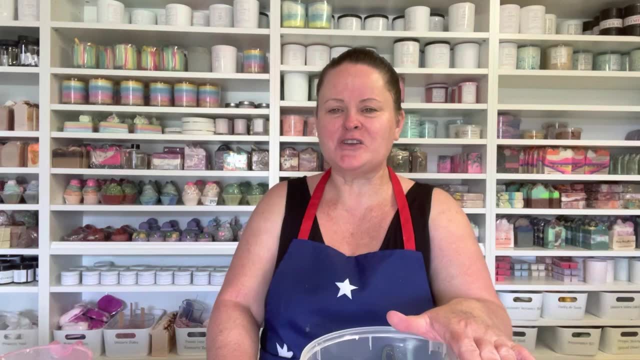 cure time or however long you're going to leave it, But, like I said, I do leave mine for around 10 months curing time. So I'm going to keep going and I will make this. We'll pop the camera down and you can see exactly what I'm doing. 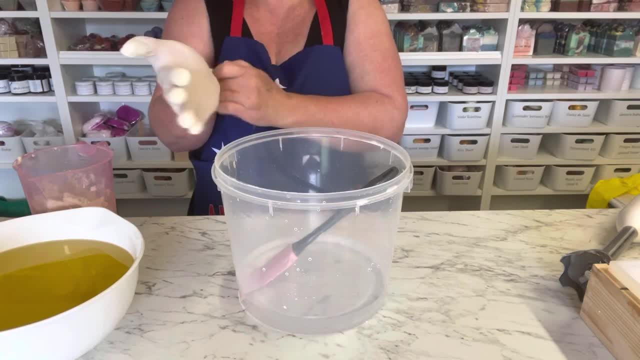 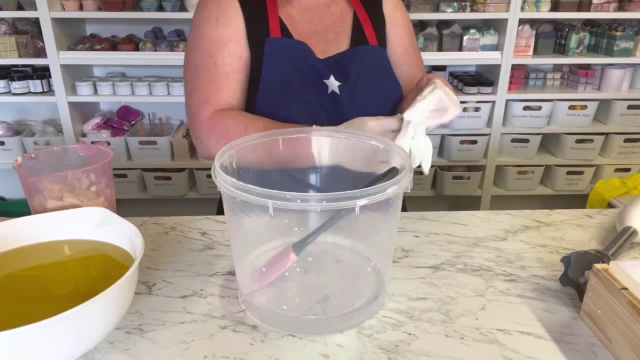 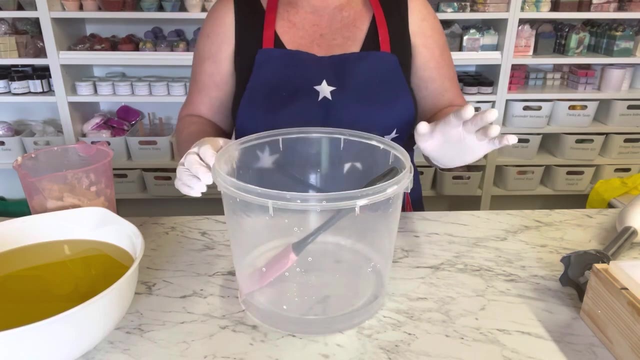 All right. so we will be putting on some gloves, of course, In here. I have already pre-mixed up all of my water, so I'm happy to tell you, you know my recipe. I don't mind at all and play around with the recipe, You know, you might just want a pure olive oil, but do remember you need to have it in. 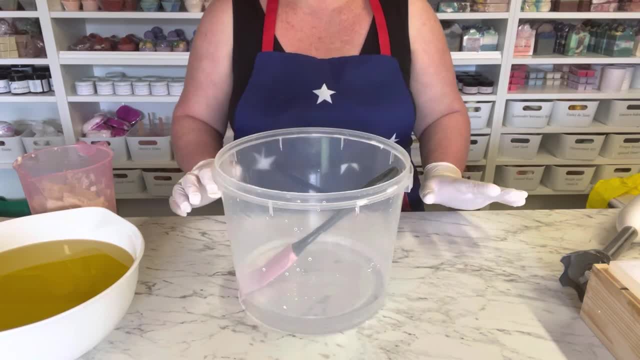 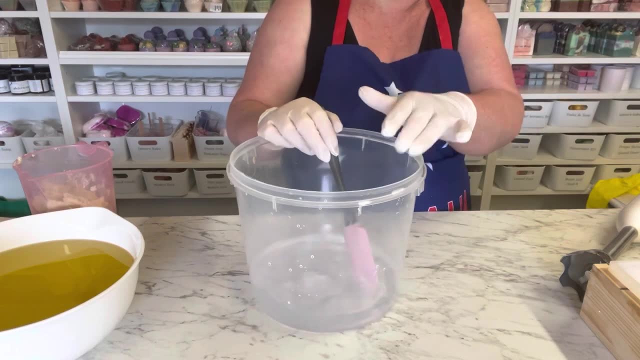 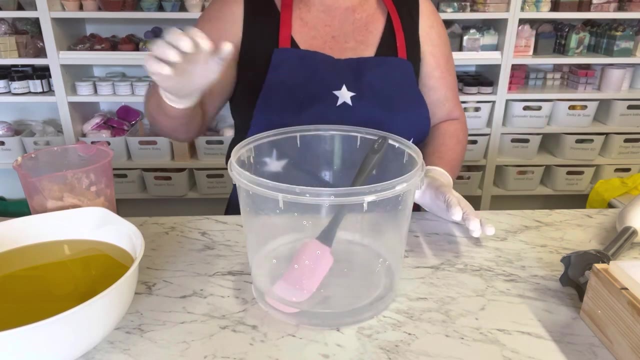 a container that you can move because it's going to, it won't harden up like normal soap in a few days time. So, anyway, in here we do have our water content, because of course we need to make this first, So this particular one here has 570 grams of water. and then of course I need 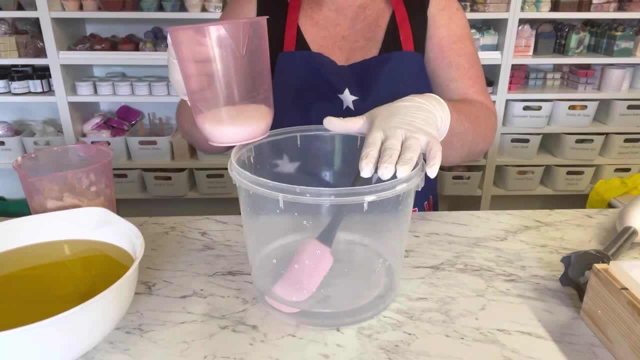 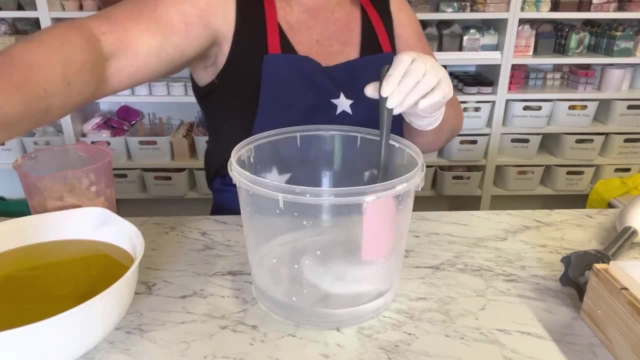 to add my sodium hydroxide because, as you know, this creates what we call lye, which is the two of these mixed together, and we're going to add 197 grams of lye in here. Always add the lye to the water, not the other way around, and do make sure that you have the right amount of water. So 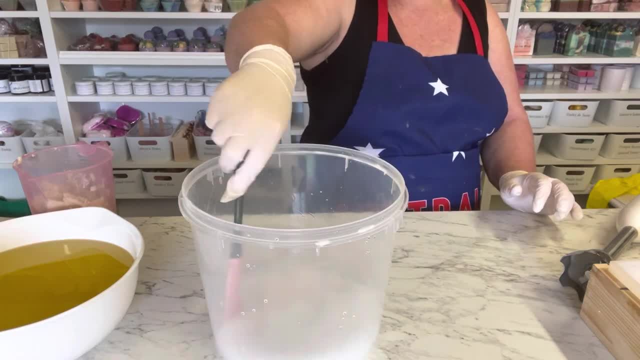 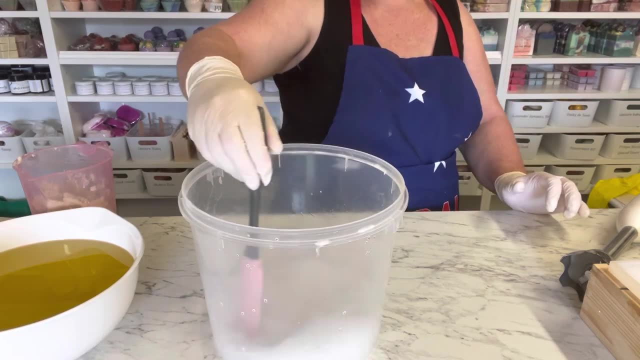 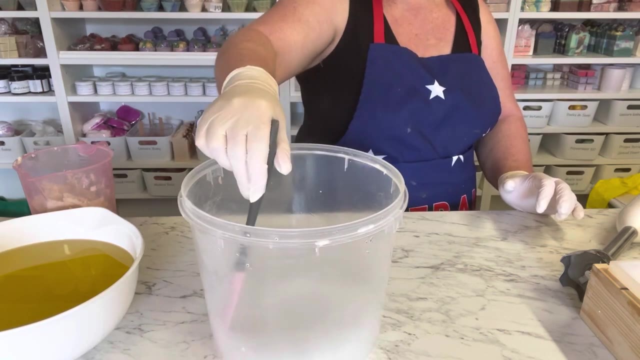 make sure you're keeping your face well away and try not to splash, Be really gentle. and you know you can usually tell when this particular mixture is ready, because you won't feel the grains running around the bottom and you know you can feel it with the spatula. It feels kind of like you know. 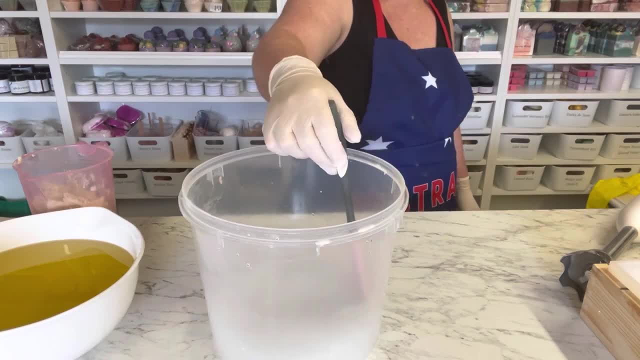 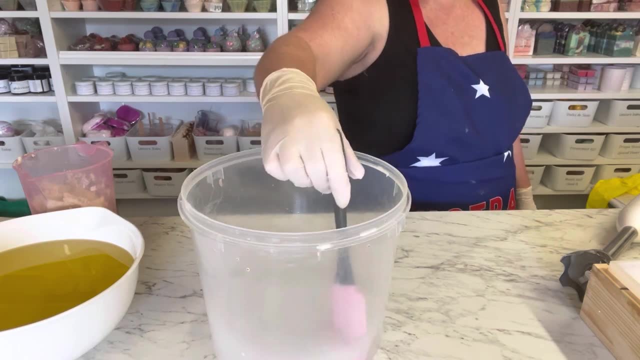 gritty sand. but once it all does its little job and it all dissolves, then you will actually know- and usually this liquid that you can see it will- the liquid will really get a little clearer. So at the moment it looks really really foggy, but you'll be able to see it's much clearer once it actually reaches. you know the point that you want. 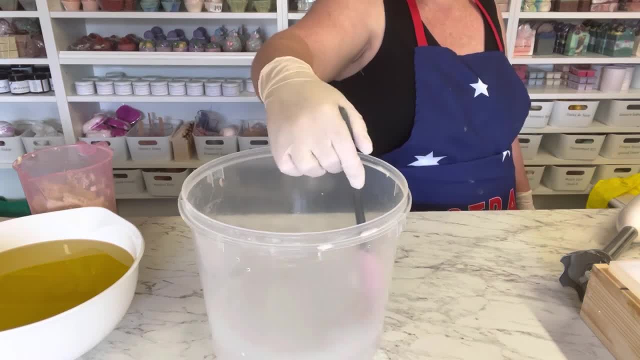 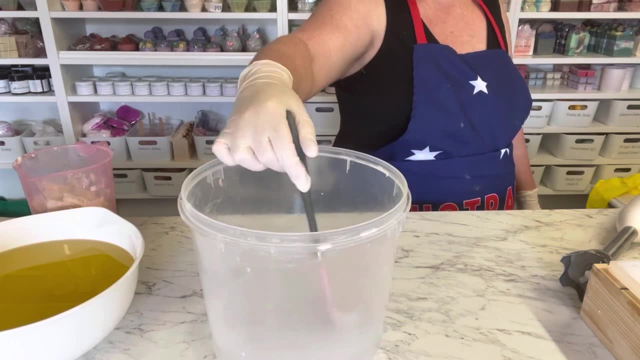 it to which, like I said, is dissolving all of the hydroxide. If you ever have hydroxide left in it and you make the soap and you see it, you need to throw it out. It means it's no good and it is way too dangerous to use. You cannot fix that. Some people may differ and give different. 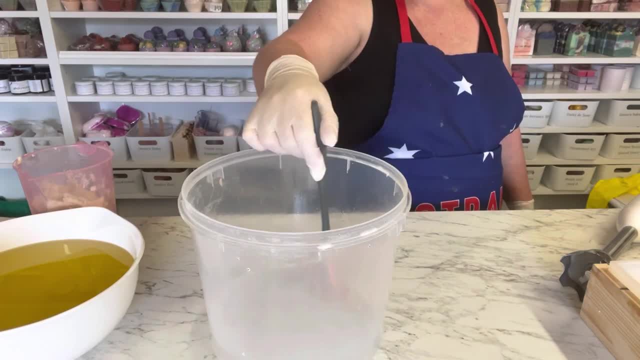 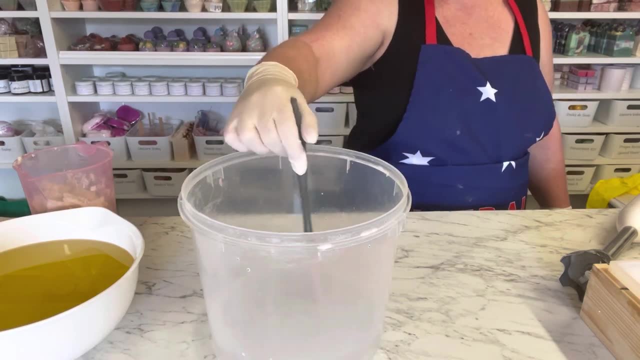 opinions, but my opinion is that it's a good idea. If you ever have hydroxide left in it and you, my opinion is throw it out. Safety is paramount when making soap. Soap is a chemical reaction, so that's the one thing people forget. It totally is a chemical reaction and you do really need to. 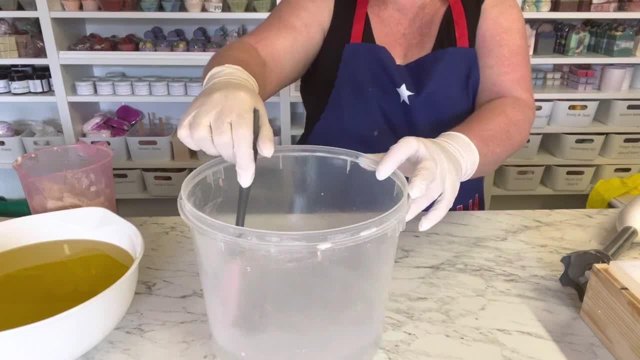 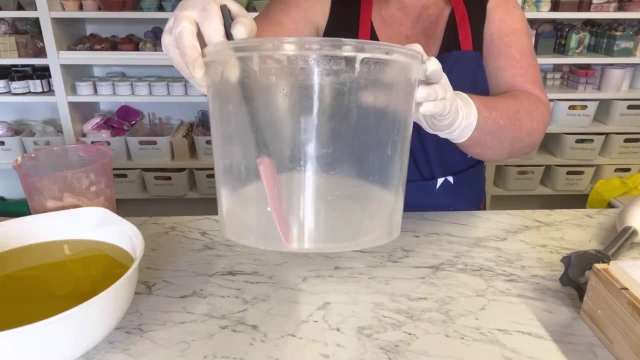 respect the process and really understand what you're making with the soap. So, anyway, we'll get going and you can see it. can you see how clear this is now like? it's really really clear. You can see the spatula through the side as well, and that's how I know this is ready to go. 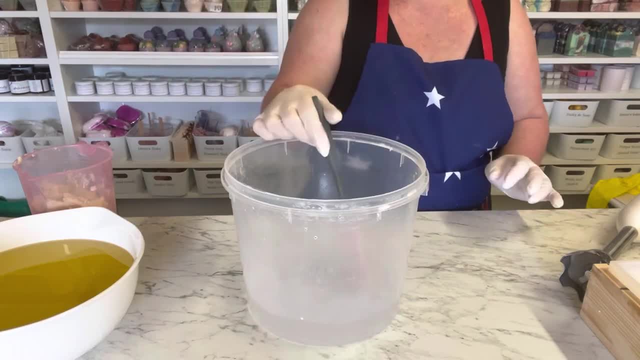 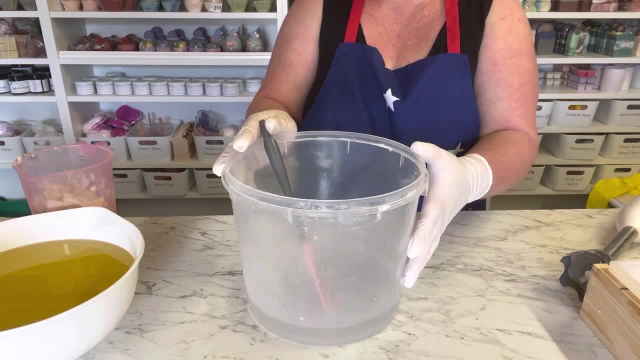 I can't see any granules and I can't feel them. so from here, because we're doing the heat transfer method, which basically means the heat of this lye, because it gets to extreme temperatures, then we are going to just simply put in our shea butter. It is sort of a warmish day today in. 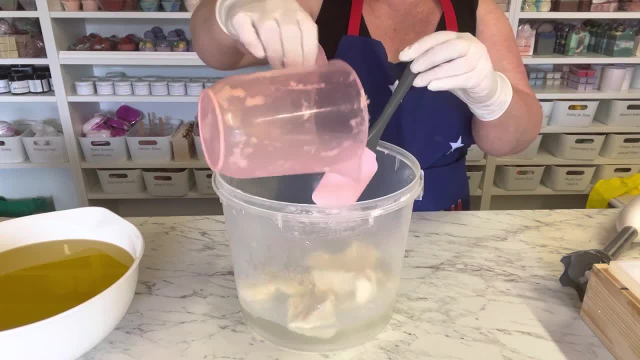 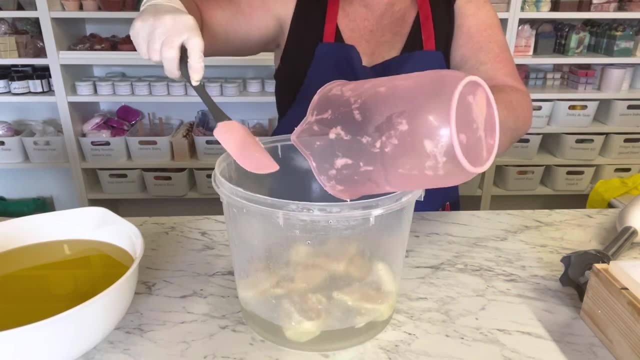 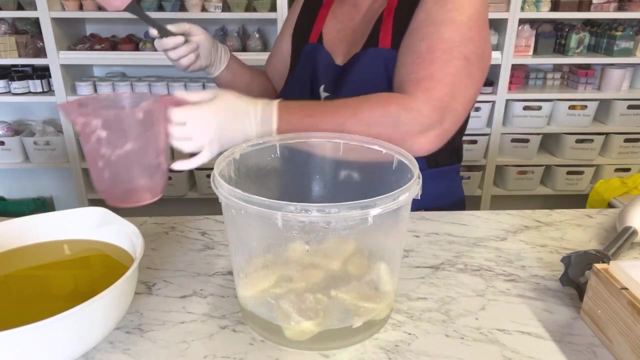 Melbourne. so I'm just going to pop it in here. Do make sure that you get everything out and try not to splash because, as we know, lye is very dangerous at this level. You know, once your soap has, you know, gone through its curing process, it's fine, it's no problem at. 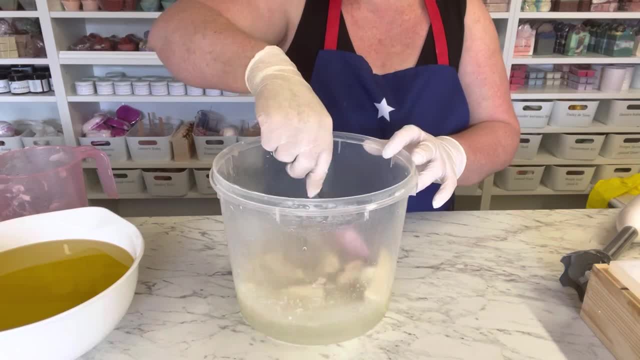 all this is how you make soap. You cannot make soap without lye, you can't. I've had lots of people say, oh, I'm going to do it without lye, and I just say the same thing: well, you can't, it's not going to. 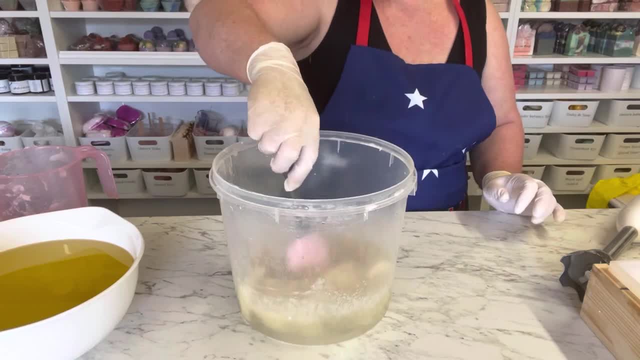 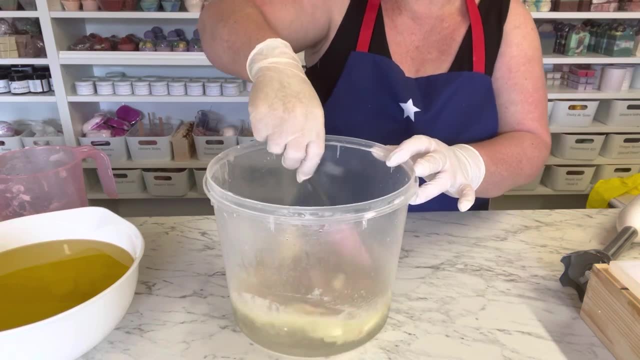 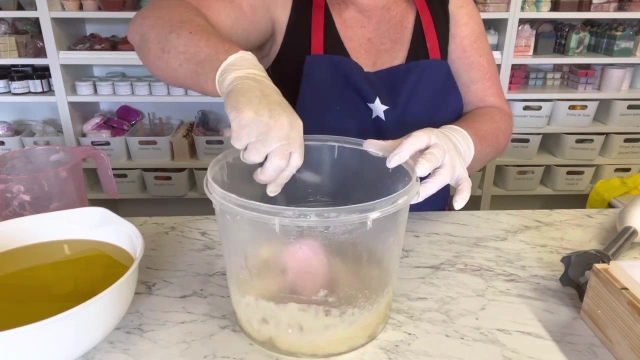 happen because it's the lye and the oils and butters mixed together and you know, and stick blended is what actually creates this. I mean, I'm sure somebody else might disagree with me, but from my understanding this is exactly how you make soap and it's how I make all my soap and sell it. 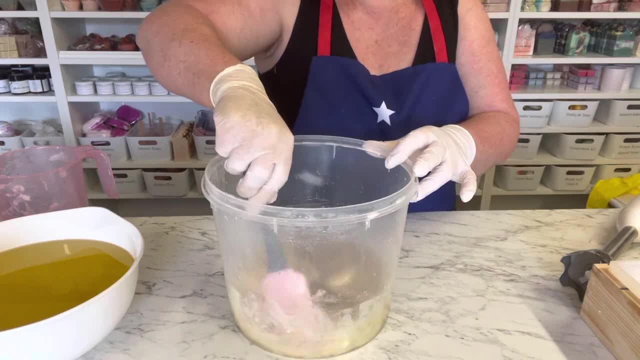 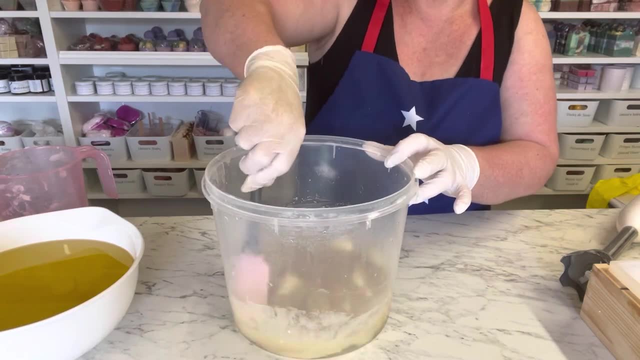 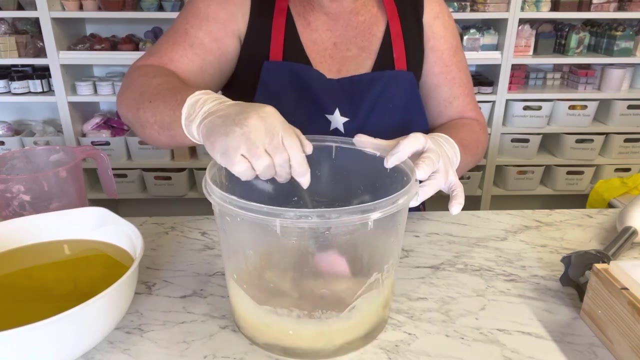 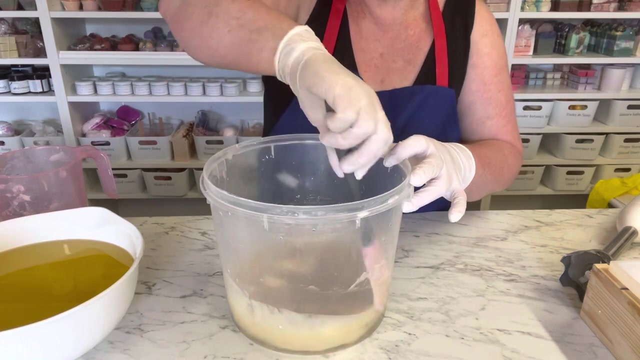 So once we mix all of this gorgeous shea butter in, then of course I'm going to add in all the olive oils. but we need to make sure that we stir all the way around here and, like I said, mix it in. So we're stirring this in. I thought let's have a chat. I mean, I don't know whether any of you guys 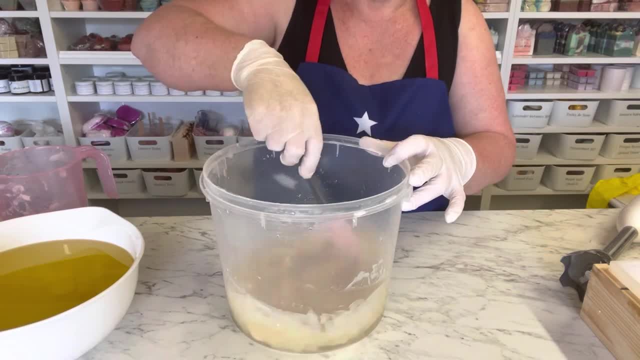 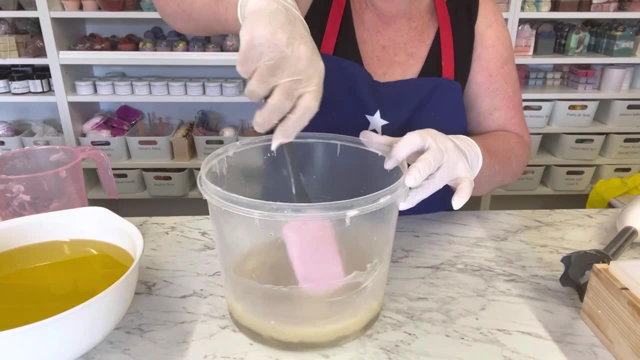 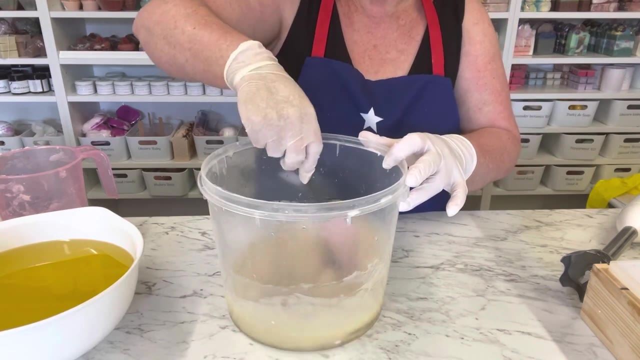 have got your immunizations for this COVID thing. that's driving me crazy. Honestly, I feel like the dog that's in the backyard never gets taken for a walk. I'm absolutely over it. I've had both of mine- my visor shots now, so thank goodness I've had them. Not that I'm saying anyone needs to or not. 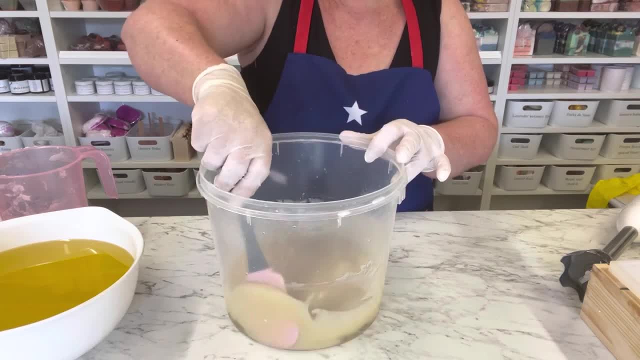 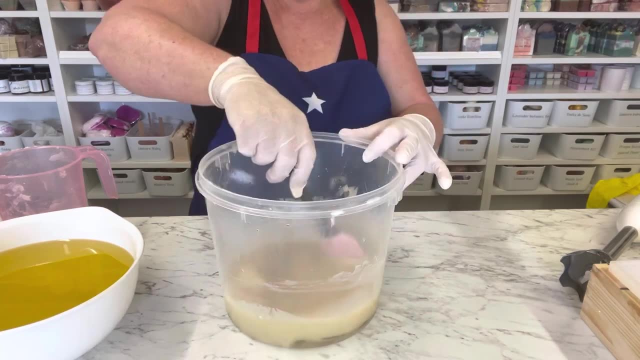 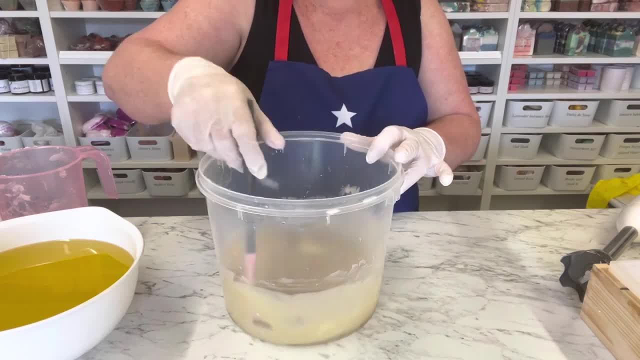 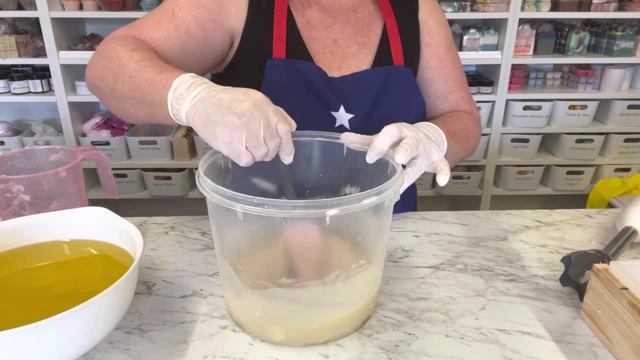 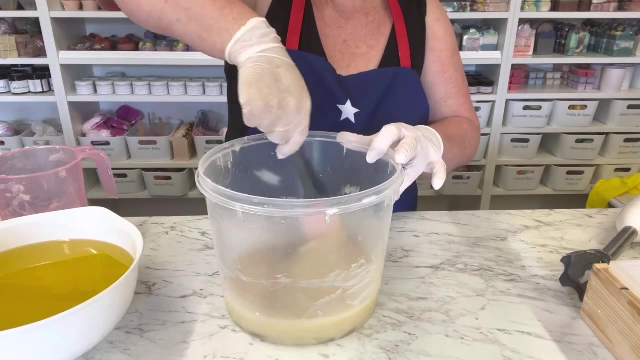 you that are new business owners, old business owners, having shops working from home, whatever, because it is so hard. So you know, if any of you are finding it hard to get your stuff into a shop, please don't panic. You know this is the hardest time to sell stuff in a shop. 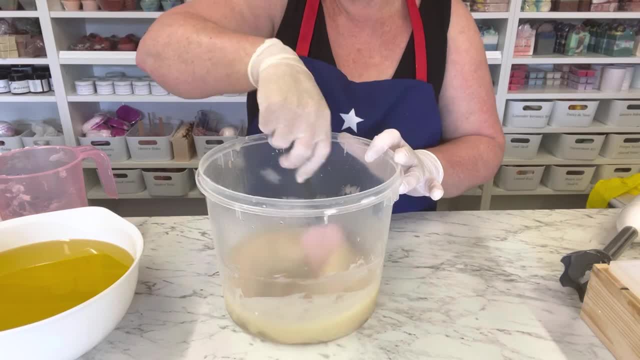 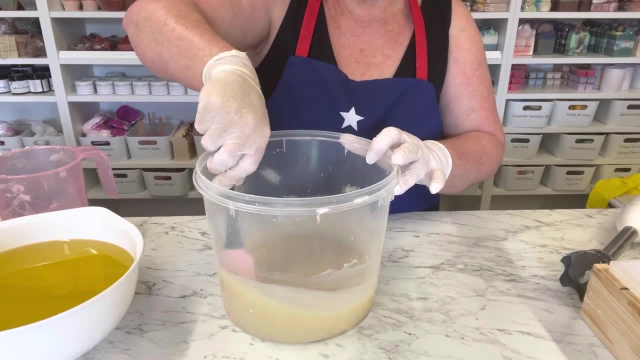 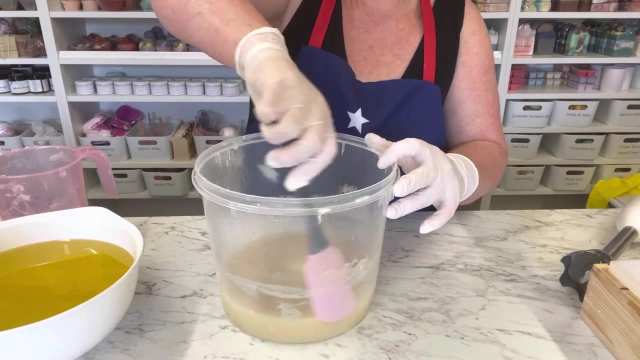 Because, of course, most of them are closed and then they're not buying anything because you know, like, for wholesale people, a lot of them aren't buying unless they're stocking up. So that's really hard too, isn't it? But online, if, if you know, you haven't started get online because 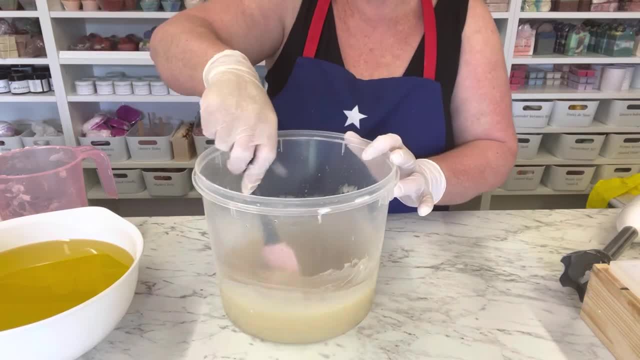 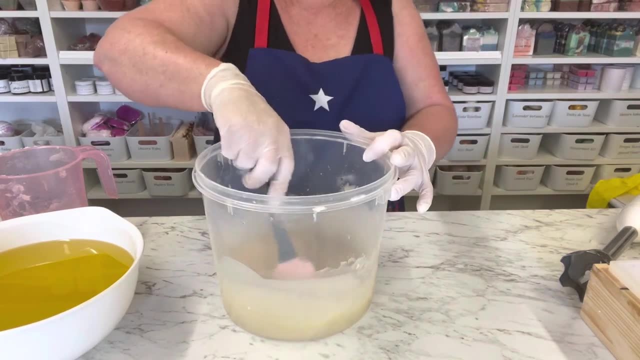 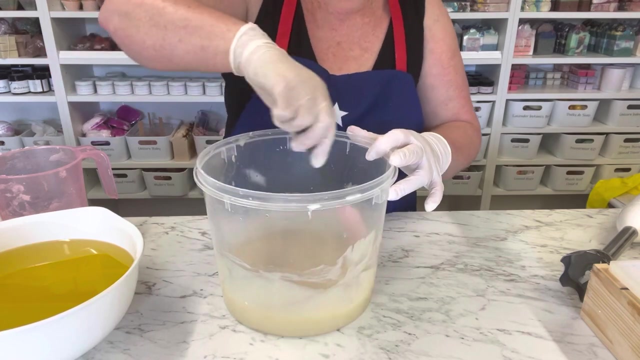 that is where everyone's buying. That is where all the money power is at the moment. So that would definitely be. my strong suggestion is: look online and, you know, see if you can get your Shopify up and going Or whatever business you want. I personally use Shopify. That's just something. takes a lot Look. 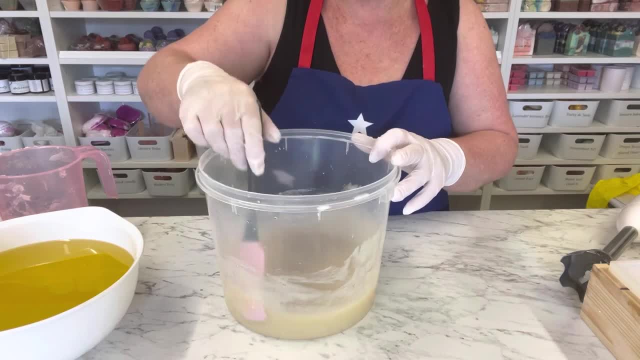 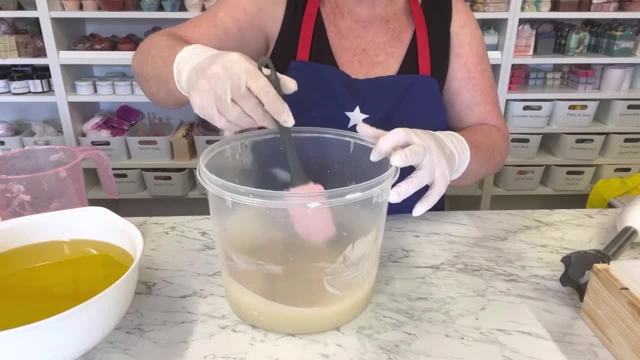 to be honest with you, it takes a lot of time to actually learn Shopify, but once you've learned it, it really is amazing because it gives you lots of analytics. You can see who's shopping, why they're not shopping, whether they put it in a cart and they don't buy it. I mean, there's just so many. 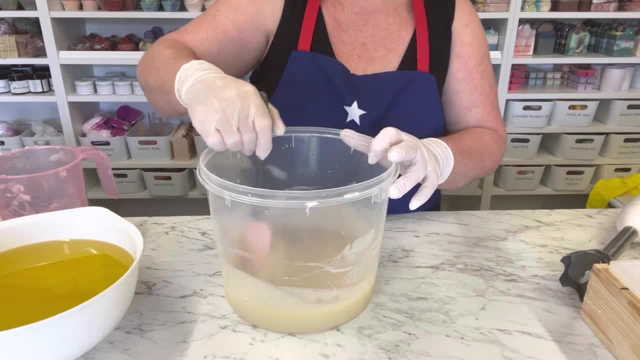 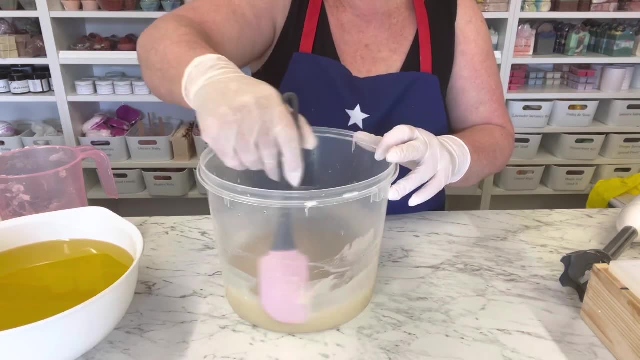 things that you can see. You can see what country people are coming to your site from the times of day. You know that the products that they favor the most, like I said, you know it tells you whether they've come back, whether they're a repeat customer. So so many things like that are so. 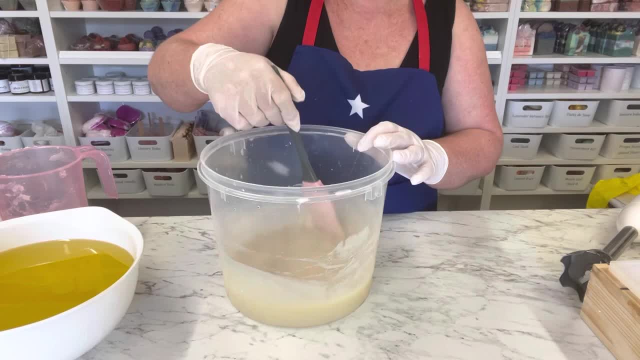 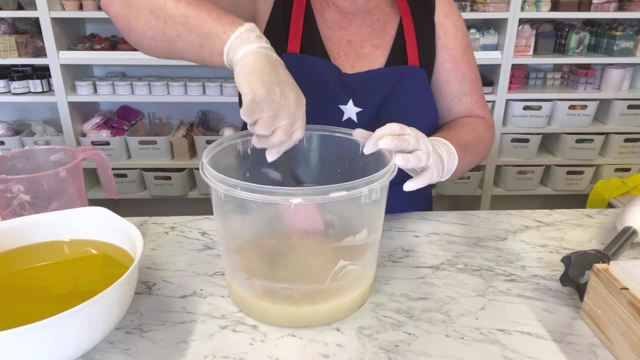 good. Plus, it's like an inventory, so because you just load all your products in and then it just keeps them all in there. But anyway, I thought I'd put that in there because I've had a few questions about Shopify lately, but maybe I'll do a video on it to help everyone. I'm not sure. 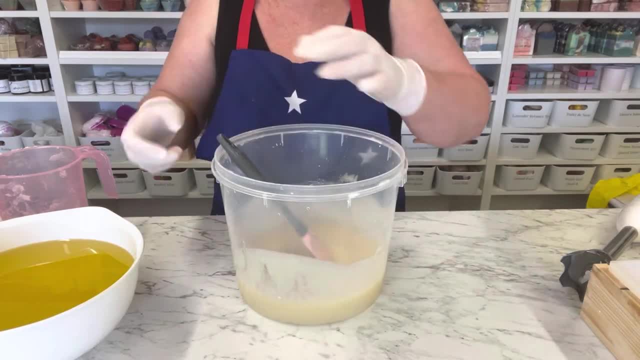 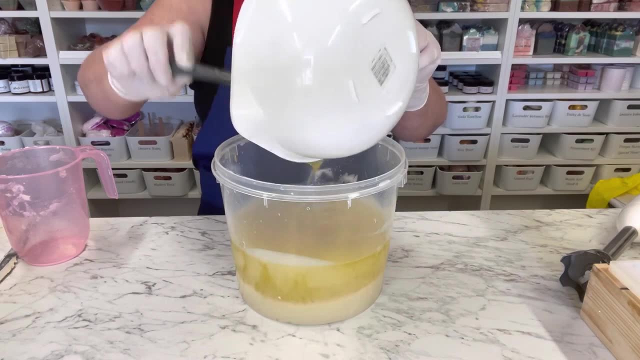 But anyway, we've mixed all this up so you can see it's all beautiful and combined, and now we will add in our olive oil. So remember, olive oil is the main content of this, because it's gorgeous, It's rich and it has lots of. 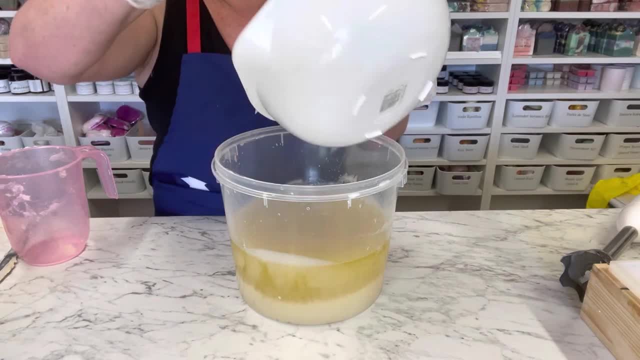 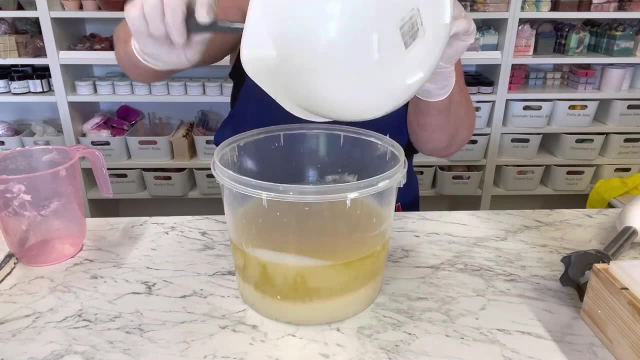 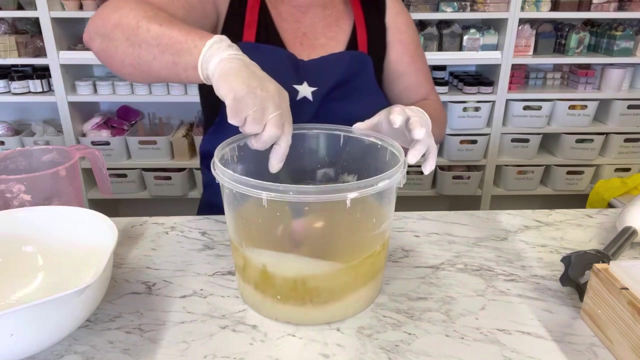 skin loving benefits. olive oil: You can get this olive oil from your local shopping center if you want to, or um, or, of course you know you can order it online. but honestly, it's just as cheap getting it from your shopping center and I just make sure I just buy some beautiful olive oil, So I buy. I 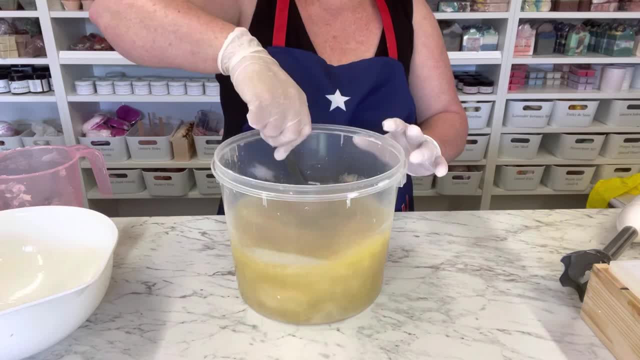 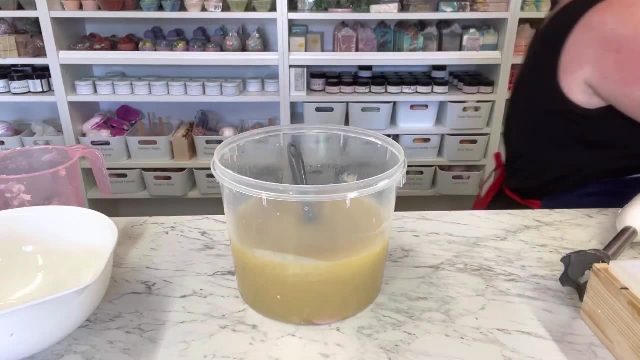 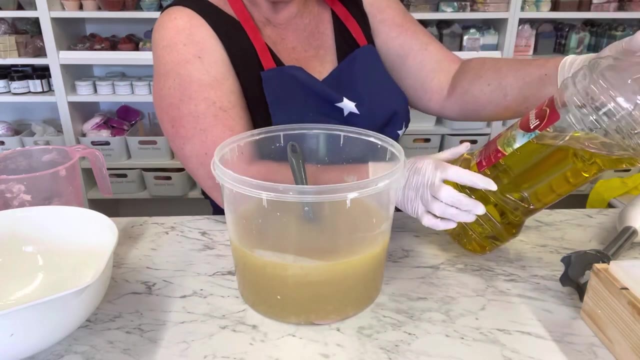 think it's an Italian brand one, the one that I'm buying, And I really like it. I had it. I was using a different brand, but, um, let me tell you- actually, I'll tell you what it is. So this is the one that I use, um, so I think it's Italian. well, it looks. 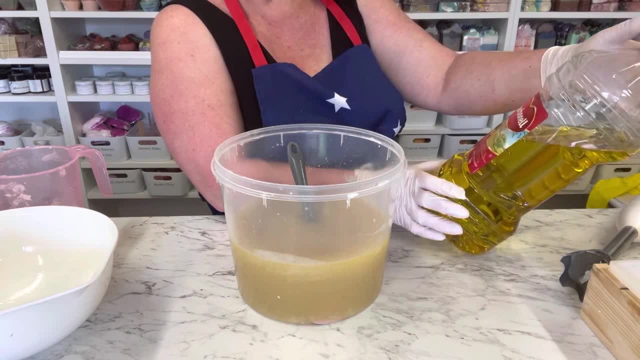 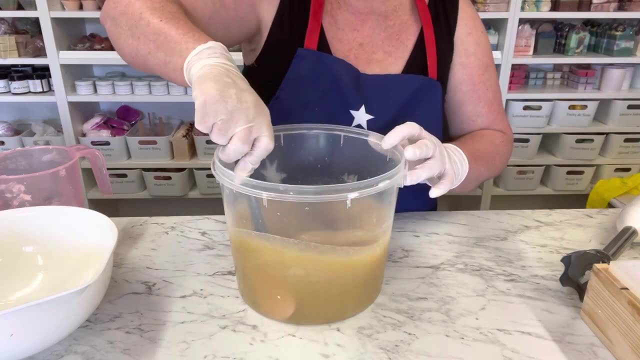 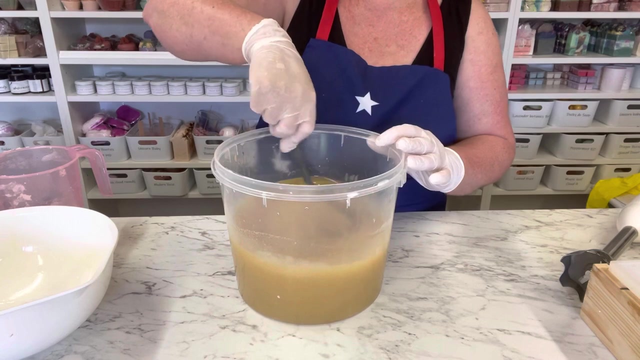 Italian to me. so I just sort of think, oh Spain, it's from, it's from Spain actually. So I buy the three liters, which is about twenty dollars for three liters, and to be honest, the ones online are a little bit lighter once it starts to cure. But for a baby soap, you don't want to be adding in. 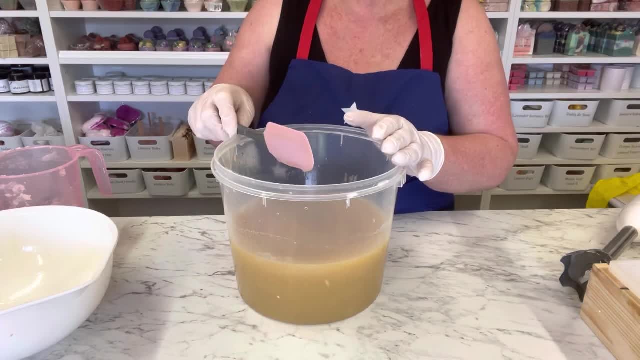 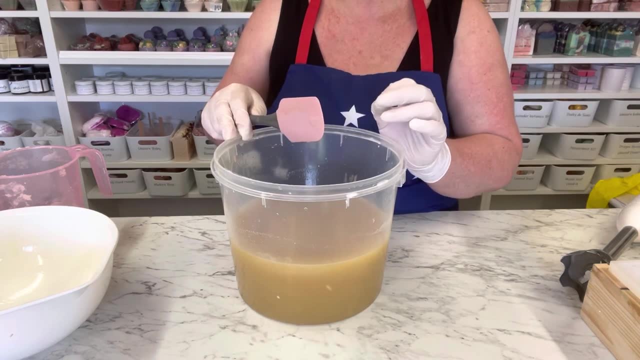 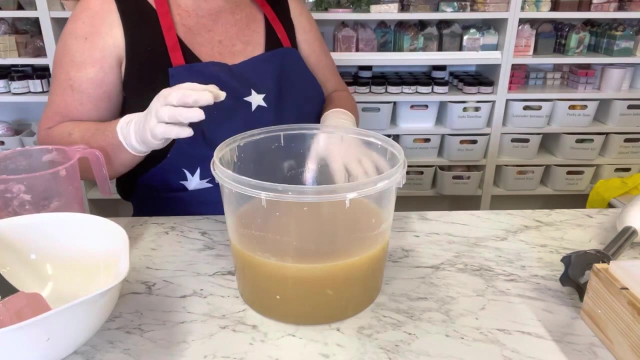 you know titanium or colors, because it's just really not that great. A baby has really sensitive skin, so you just have to keep their skin looking gorgeous, And the only thing I usually add in is a couple drops of um essential oil in lavender. So I forgot that bit, didn't I? So I'll just go and grab. 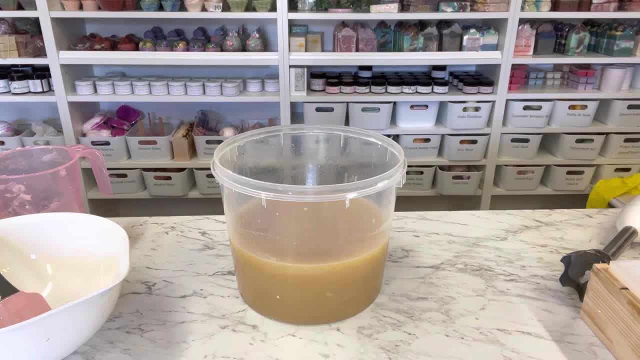 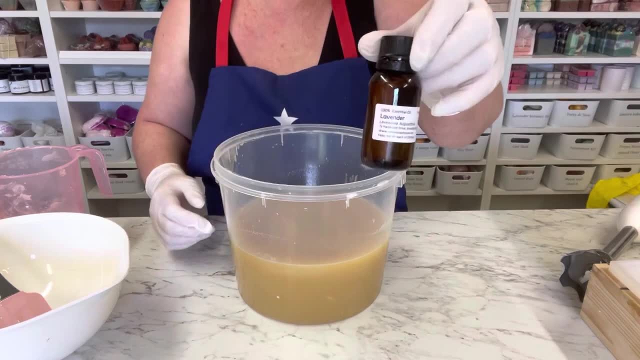 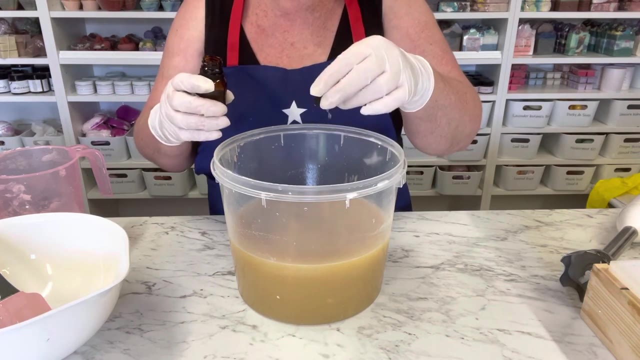 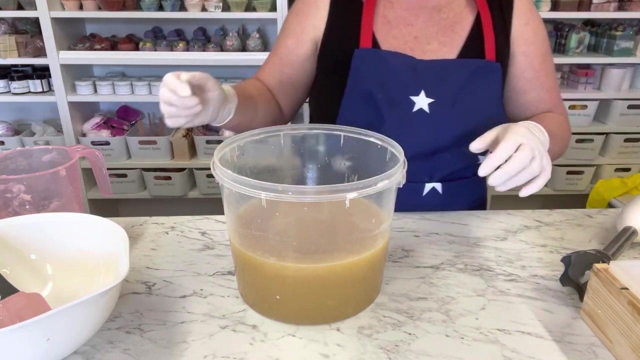 it. So the lavender I'm using this is actually from Robin's Soap House and, like I said, I only add, so I just put a little bit in the lid. I mean, honestly, you can see that's just a few drops. it's like about five drops in this whole thing, And then I'm going to be putting it into my 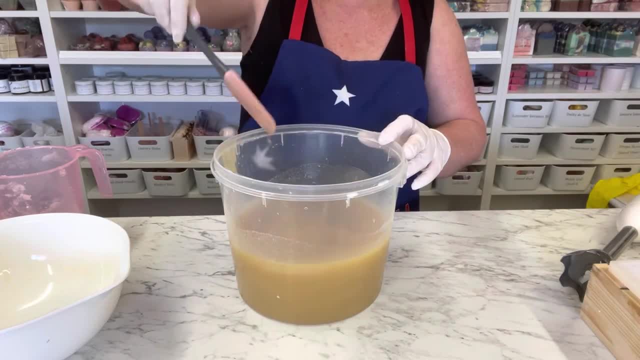 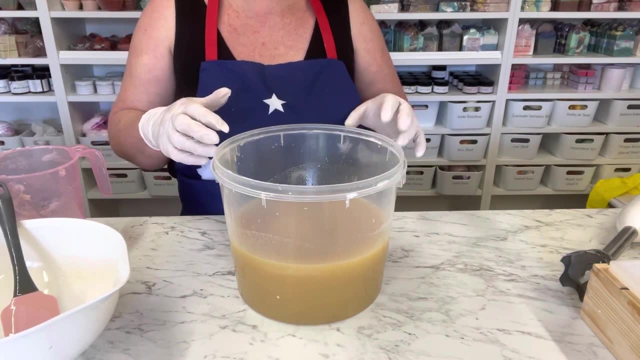 gorgeous container. but before that, of course, we all know the next step: we need to um blend it. Now, do remember when you're making baby soap, because it doesn't have all the fats in it. it's not going to be really thick, it's going to be quite watery, but you just need to make sure it. 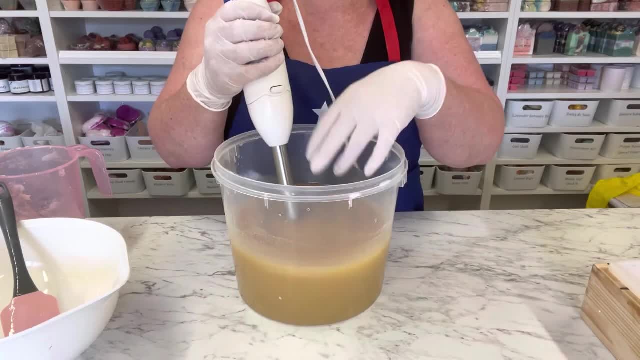 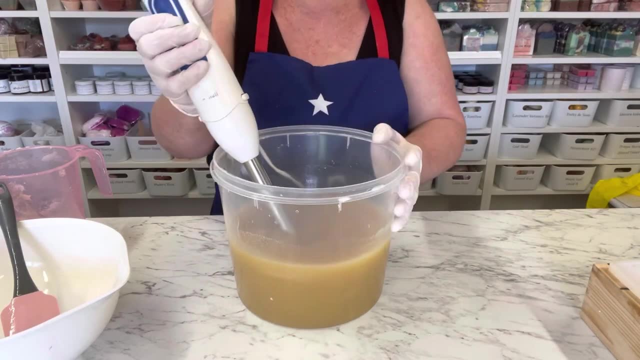 comes to trace, And if you don't know what that means, it means when you blend it and you kind of wave this over the top, the little droplets should leave like a little line or a trace on top, and that's what the trace is called. 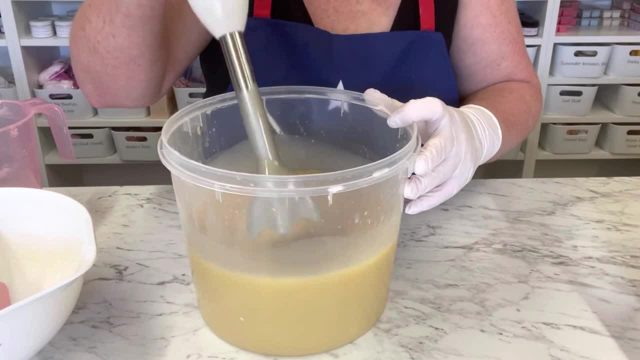 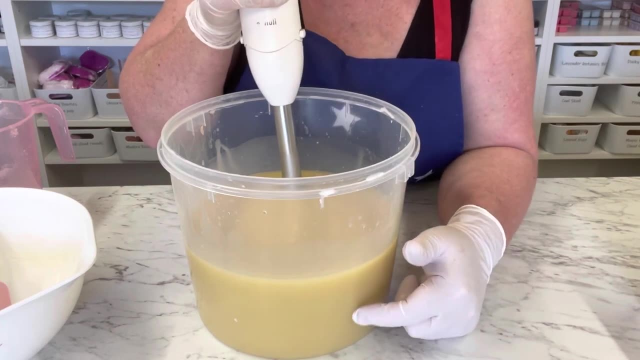 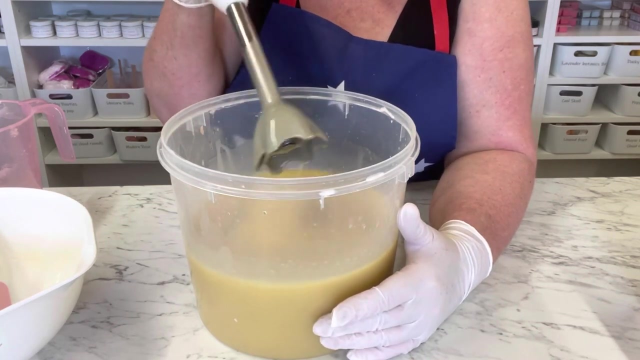 And two, when you're actually making soap, I thought I'd tell you. usually you can see from the outside of the bucket if you get oil sitting on the top, that means it's not blended enough. So you know, you'll see it kind of separating and that is an easy way to tell. I'm just going to give this a. 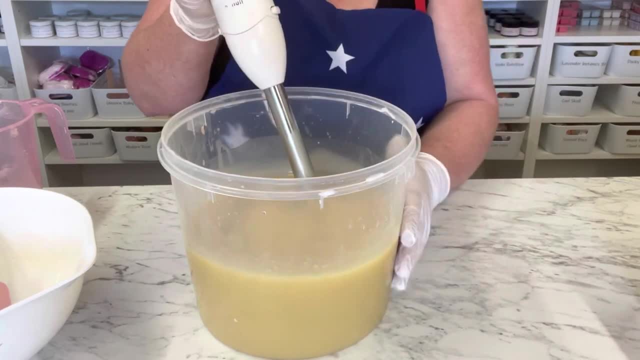 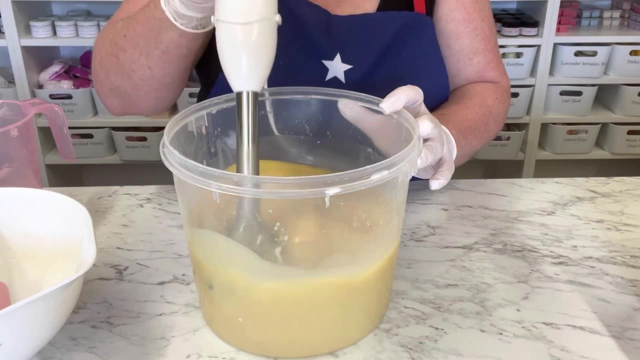 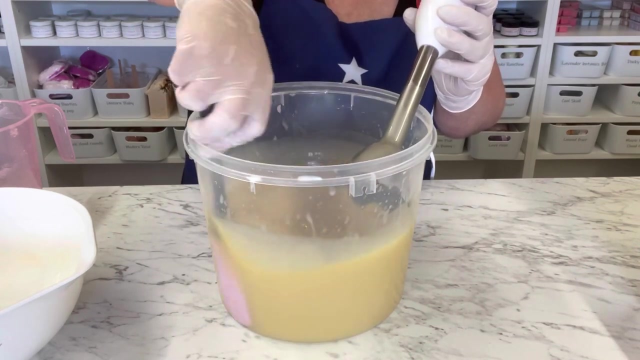 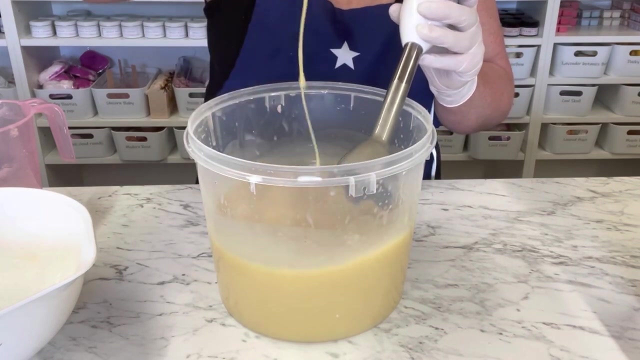 little bit more of a blend and then we will pour it into the container. So we just mix it around and make sure it's done its thing, Like I said. you know, please don't think this is going to get um thick, because it's really not. I mean, you can see how watery that still is. 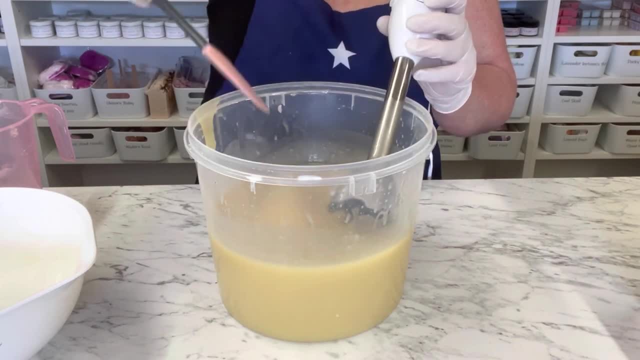 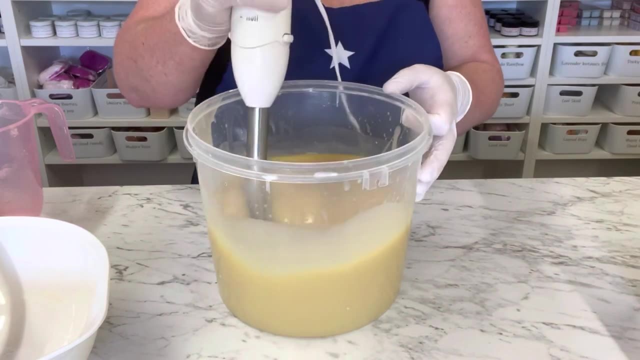 but it's fine. I can see that it's not separating. It's more than fine to go and pop this in. So we will just give this a little bit more of a stir and then I'm going to pop it in to this, which is the container. So I'm just going to give this a little bit more of a stir and then 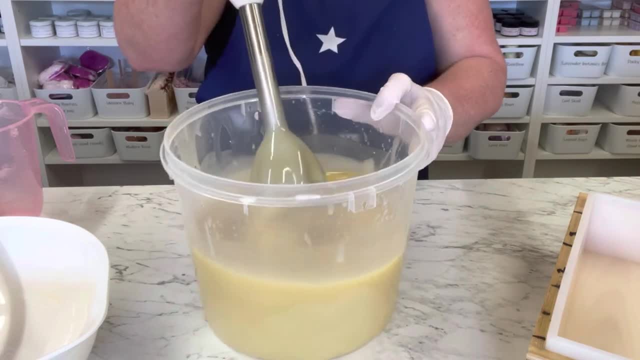 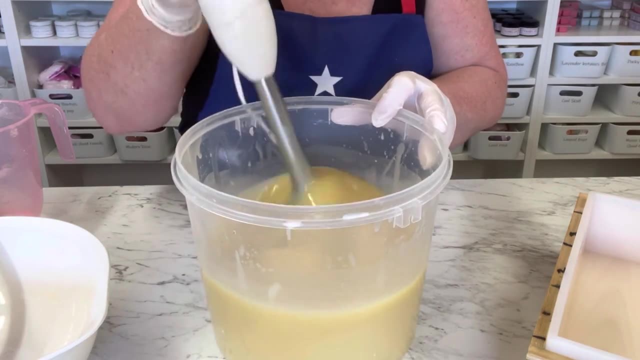 I'm going to pop this in to this, which is the container that I'm popping it in. I stir this around. so when you actually do this and you- I don't know whether you can see from the camera, but you'll have like little tiny baby lines that come on top, which I can definitely see. 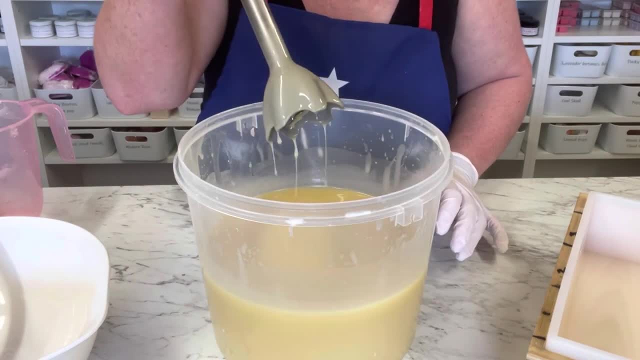 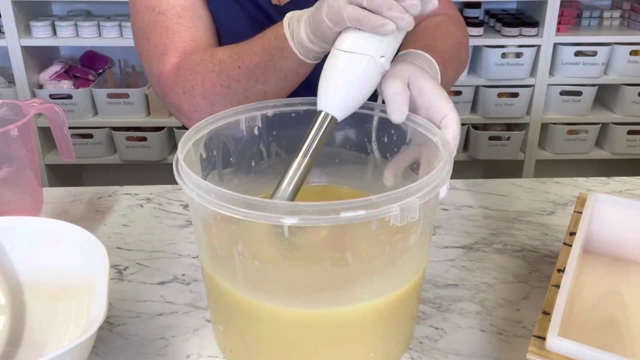 a very, very slight tracing line and then I know that this is all good and it's already. you can see that it's not separating, It's quite mixed together. So, yeah, so, and, like I said, baby soap isn't different to most others, and now we will just pour it into this. 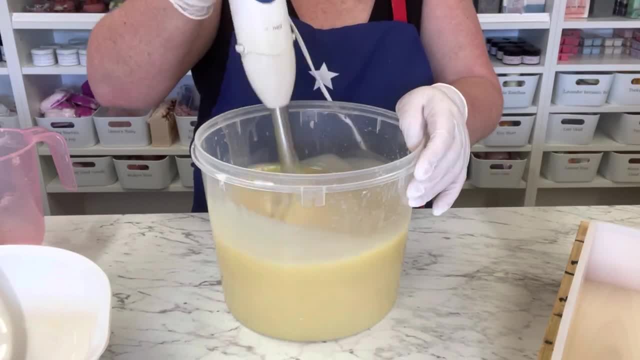 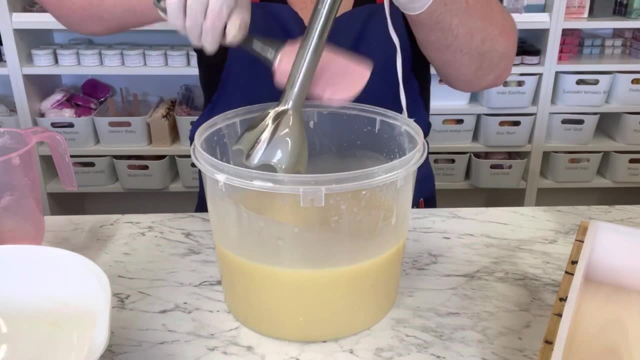 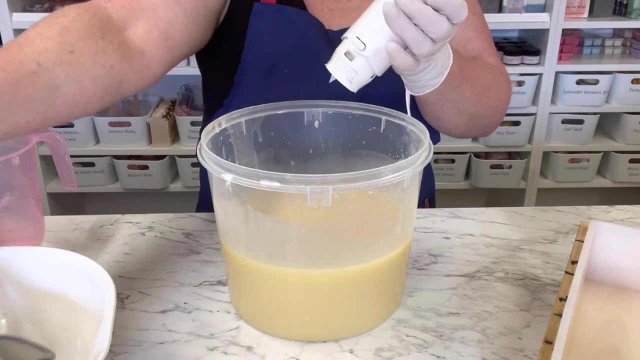 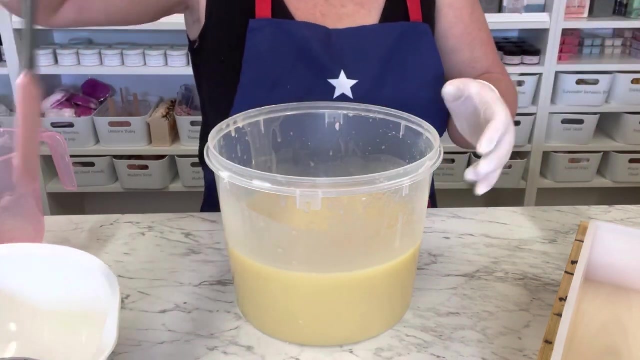 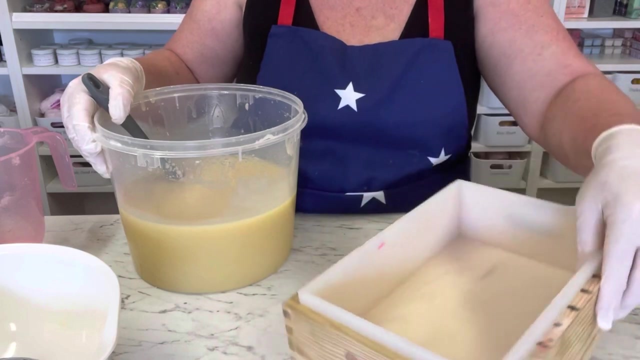 container. all right, as we know, it is all ready. here is my container I have. all right, as we know, it is all ready. here is my. have drawn a tiny little pink line, if you can see there, because I know I don't want it to go any. 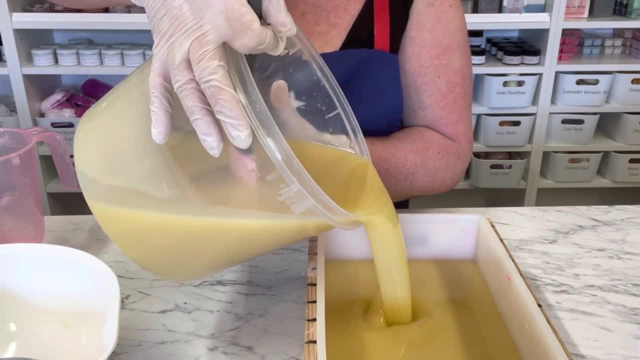 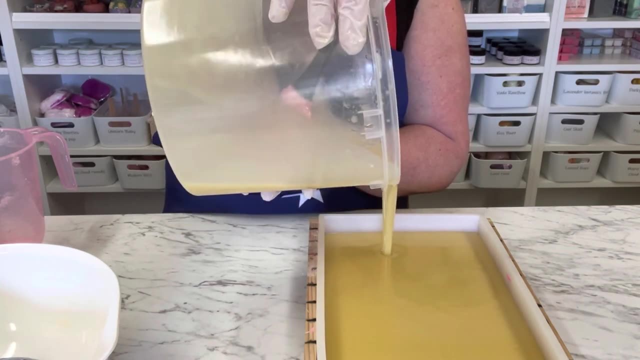 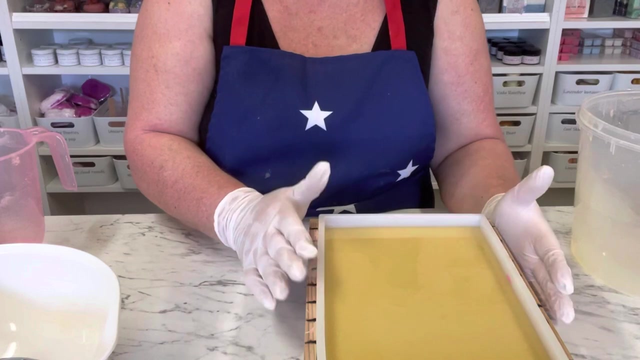 higher than that, because then this will fit into my baby box. so I just know that it cannot go any higher than that. so it will fit into the boxes and I think that is pretty much perfect. so, with this, the one thing that you're going to notice with this is you definitely can't do the swirls, or 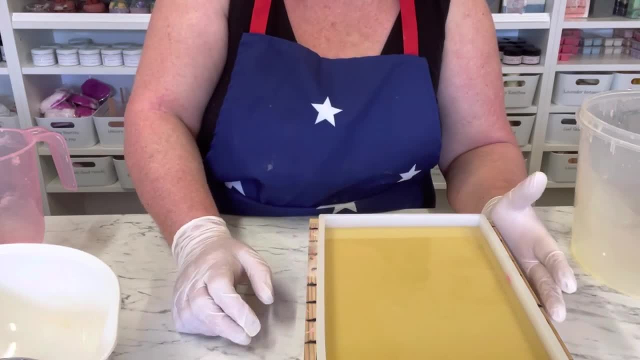 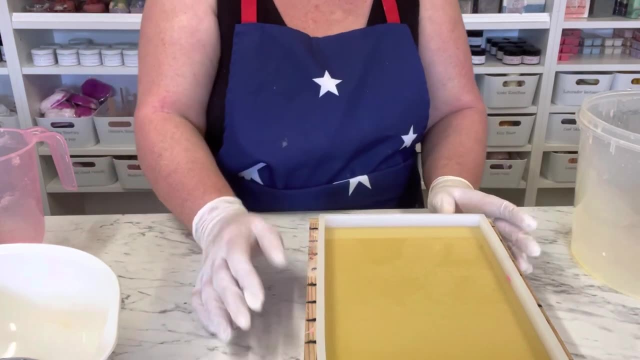 anything, you'd have to leave it for hours before you could come back and do it. So I'm going to come back, but if you wanted to do a bit of a pattern on the top, which I have in the past, just leave it for a while and come back in maybe 40 minutes. it will take a long time, but as you can, 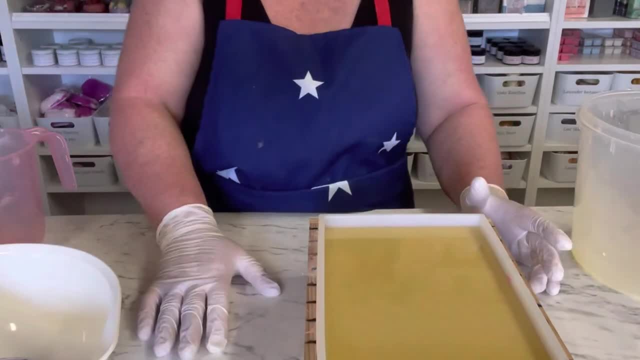 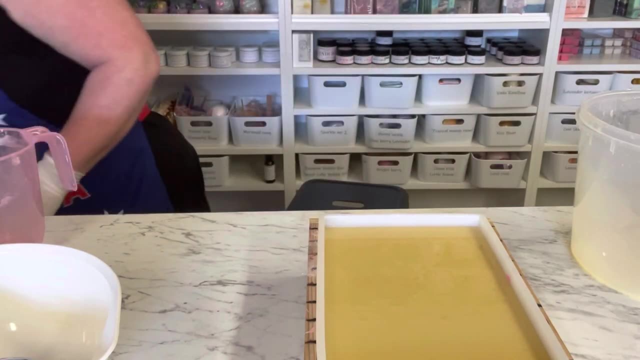 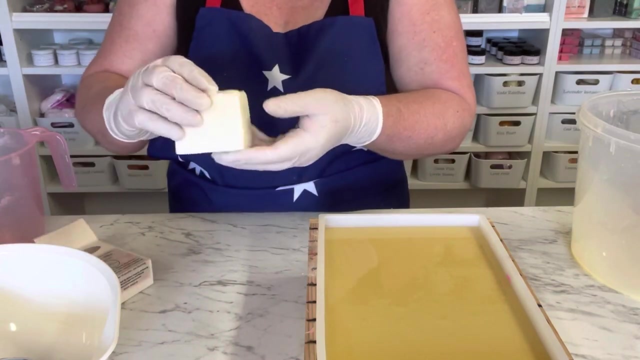 see, it looks really, really gorgeous, doesn't it? you won't see the cut of this. I'm sorry, but you definitely will not. but I can actually show you one that I've already got curing. so when I make my baby soaps, I pop them in these little boxes and I'll open one up so you can see. and this is what it looks like in here. 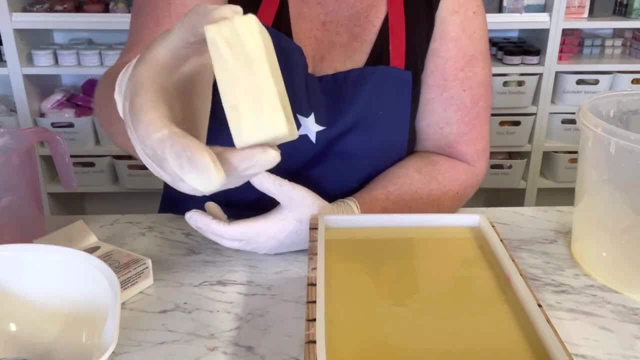 So this is the baby soap that I've made quite some time ago and, um, yeah, it looks gorgeous. sometimes I've noticed that you will see a tiny discoloration because of the high oil content, but that's all a part of having this particular soap, so, but generally you don't. but you know, sometimes you will just to let you know. anyway, hope you've liked this video, guys. if you do, make sure you give me a massive, big thumbs up and everyone. stay safe, go for a walk and I'll see you in the next one. Bye, bye.